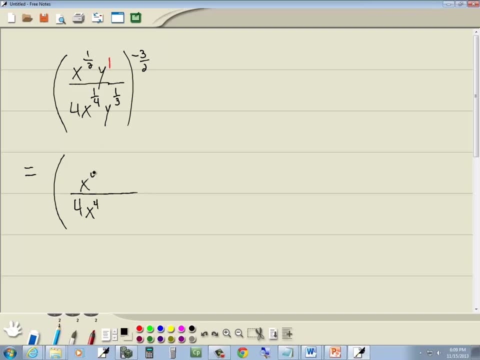 So we're going to rewrite each one with that denominator. Now this bottom part already has it, so that stays one-fourth Top part, though we multiply this by two, so we multiply the top part by two, so one-half becomes two-fourths. 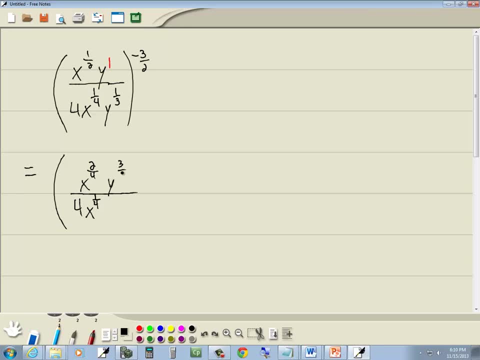 Now the one. we can rewrite that as y to the three over three, And then this is y to the three over three, And then this is y to the three over three, And then this is y to the three over three. Whenever you have a first power like that, then your other denominator is a common denominator and the easiest way to rewrite one is three over three. 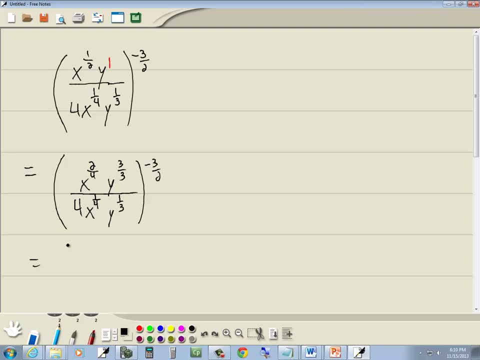 Okay, now we can do some simplifying. Four stays down here. We have x to a power over x to a power, So subtract the smaller exponent from the larger one. This is for the x's. So we've got two-fourths minus one-fourths. 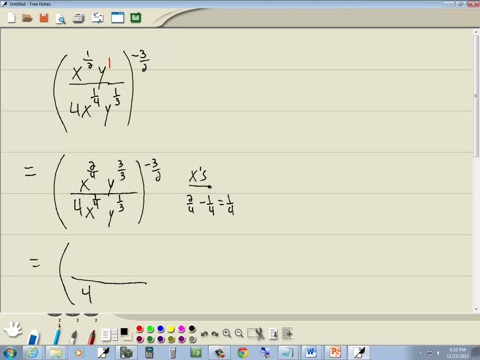 So we're going to have x to the one-fourth where our larger exponent was, which is up on top. Now our y's. We've got y to the three-thirds over y to the one-third, So we're going to subtract the smaller exponent from the larger one. 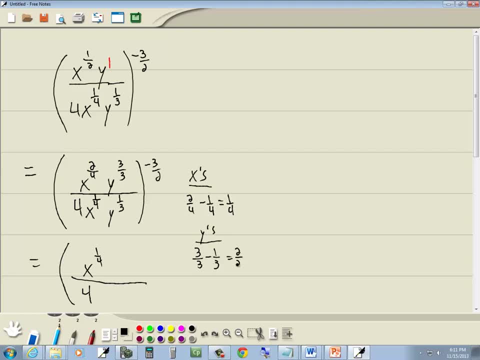 So we've got three-thirds minus one-third, which gives us two-thirds. So we're going to have y to the two-thirds where our larger exponent was, which is on top. Okay, still following the order of operations, There's nothing left to do inside of the parentheses. 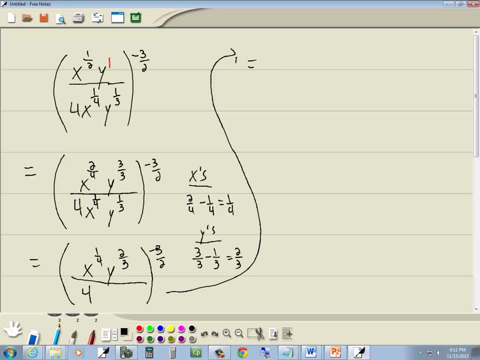 So we'll handle the exponent on the outside and it's a negative exponent. Well, whenever you have a single fraction equal to a negative exponent, you can flip the fraction, take a reciprocal of it, So it becomes four over x to the one-fourth, y to the two-thirds, and then a sign of your exponent changes. 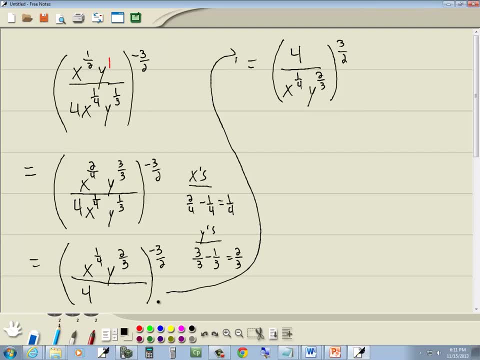 So it becomes a. It's a positive three-halves. Okay, Now, if everything inside of your parentheses is a multiplication or division and you raise it into a power, you're going to take everything to that power. So we're going to take the four to the three-halves power. 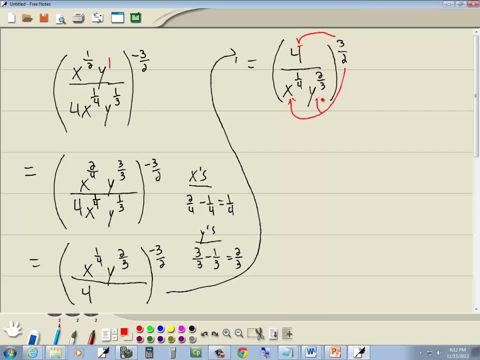 We'll take the x to the one-fourth to the three-halves power, And we'll take the y to the two-thirds to the three-halves power. Okay, So we're going to have four to the three-halves over x to the one-fourth. 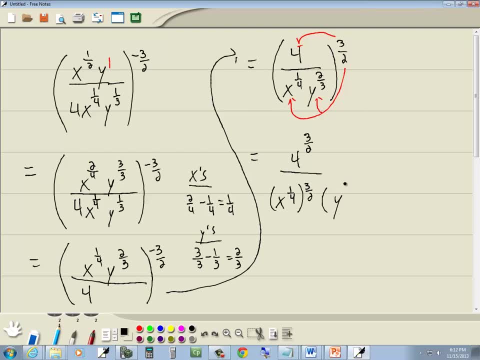 To the three-halves power And y to the two-thirds, to the three-halves power. Well, up on top we've got a number to a fractional power and the numerator is greater than one. So we want to split that up. 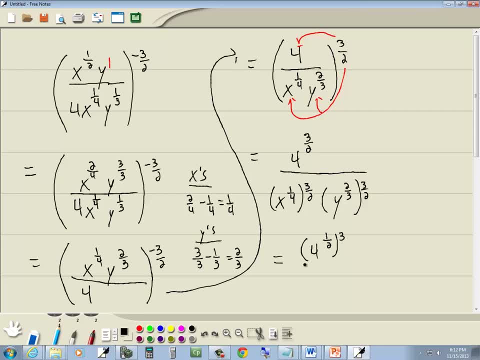 We want to put the numerator, the three, on the outside of the set of parentheses, Now down below this, right here. there's nothing to cancel here, So I can go ahead and just multiply those together. One times three is three. 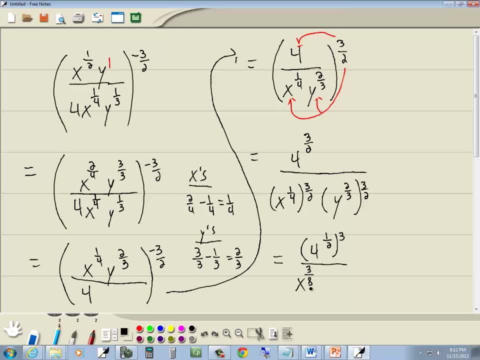 Four times two is eight, So that becomes x to the three-eighths. Now for the y's over here, though. this got two here, two here, So those two's going to cancel. We got a three here. we got a three here. 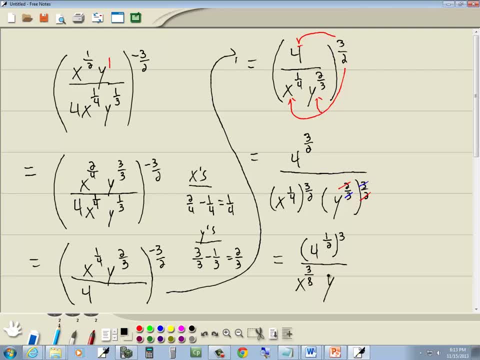 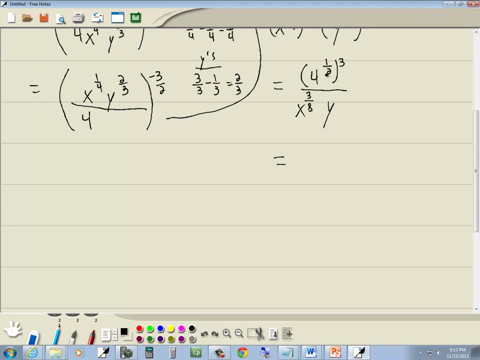 So those three's going to cancel. So that leaves us with a single y: Okay. Well, the bottom part's simplified as much as we can, but let's go back to the top Four, to the one-half. we're going to rewrite that in radical form. 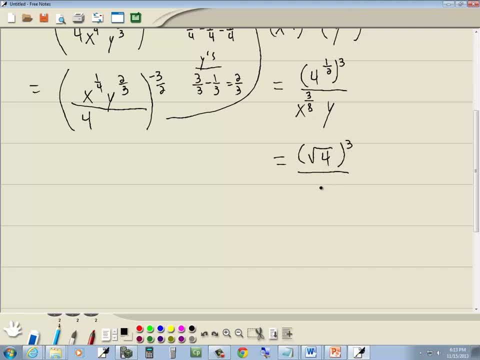 That'd be square root of four. So the third power. We've got x to the three-eighths y Now square root of four. four is two times two, So square root of four is two. So that's two to the third over x to the three-eighths y. 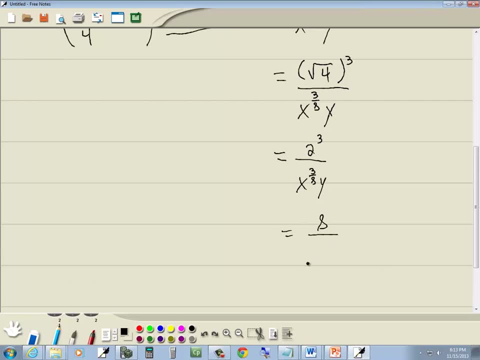 And two to the third gives us eight. So we're going to have eight over x to the three-eighths y, And that's our answer. 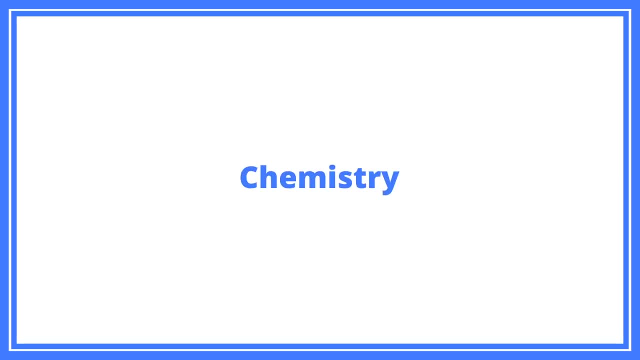 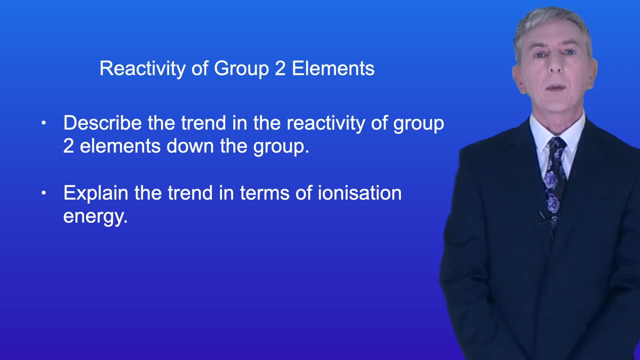 Hi and welcome back to Free Science Lessons. By the end of this video you should be able to describe the trend in the reactivity of group two elements down the group. You should then be able to explain the trend in terms of ionization energy. I'm showing you here. 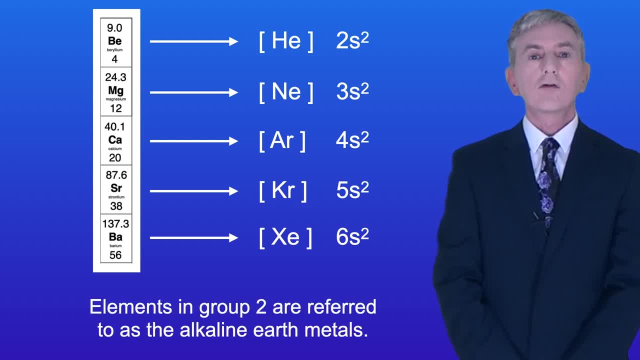 the first five elements in group two. Elements in group two are referred to as the alkaline earth metals, and a key idea you need to remember is that alkaline earth metals are reactive. Now, all of the elements in group two have two electrons in the S subshell of their outer.